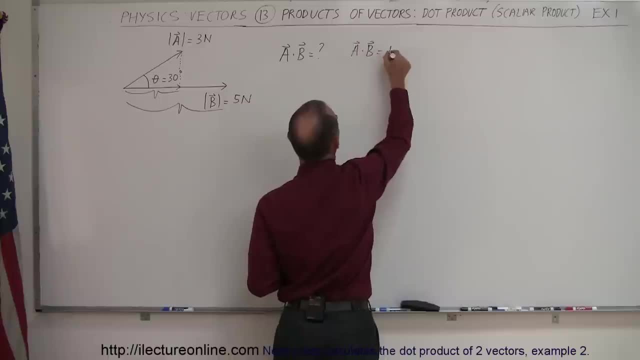 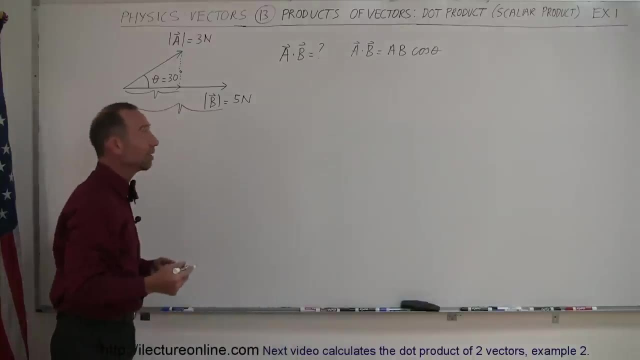 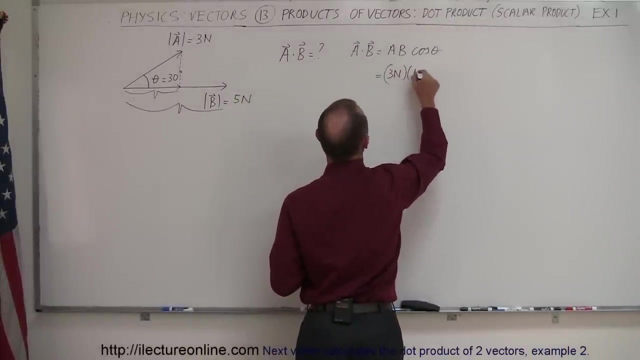 So A dot B is equal to the magnitude of A times the magnitude of B, times the cosine of the angle between them. Now, in this case I was given the magnitude of A and B, so that makes it very straightforward. So this would be equal to 3 newtons times 5 newtons times the cosine of 30 degrees. 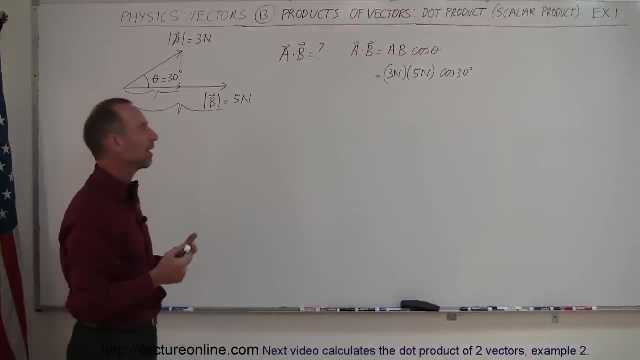 Now notice: the units are going to be newton squared, which really doesn't have much of a meaning. But this is just a little bit of a equation. This is a theoretical problem, so we don't have to really worry. I'm looking for my calculator here. 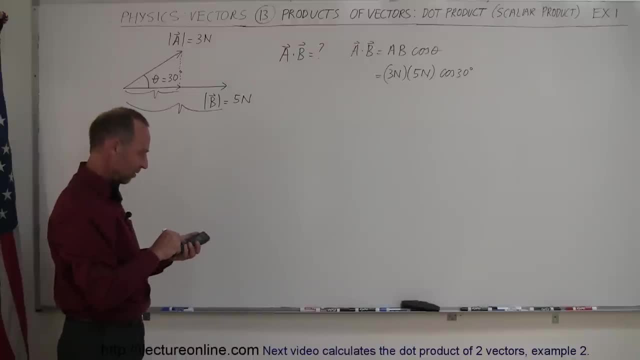 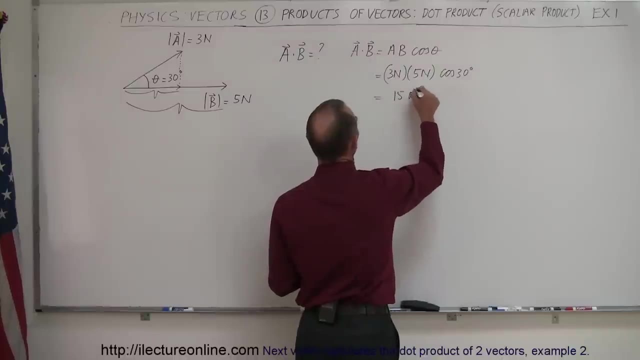 about the units there. So the cosine of 30 degrees is 0.866 and then we multiply so this is equal to 15 newton squared times 0.866.. And so that would be times 15 equals. that would be rounded off to: 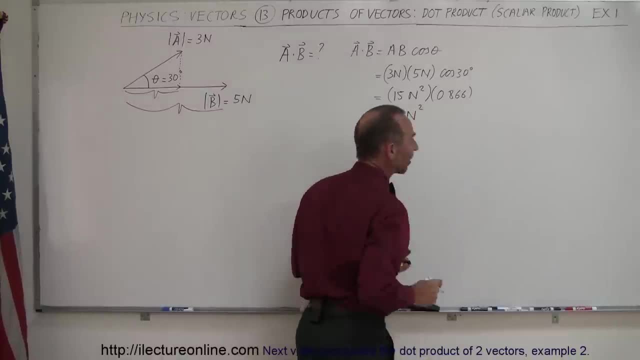 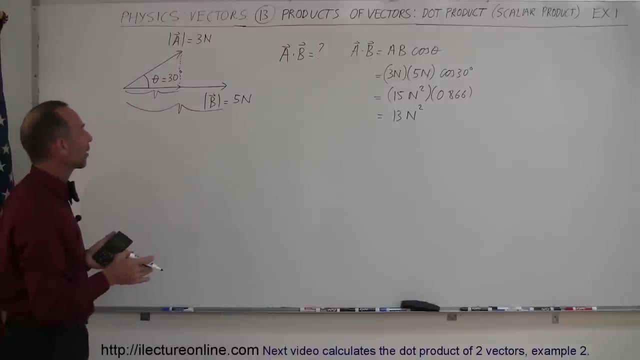 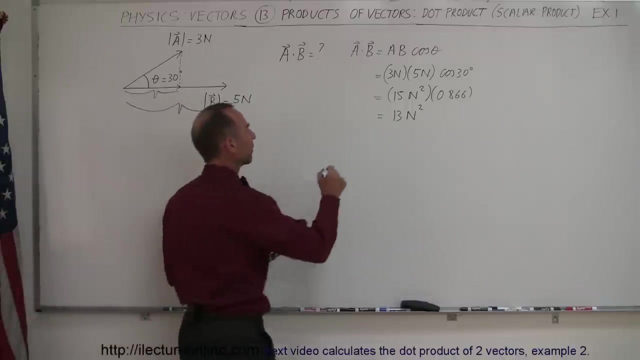 two significant figures would be 13 newton squared. Now say again: don't worry about the newton squared. normally in physics we don't really find the product, the dot product, the two force vectors. So that's why I end up with these funny units. But remember also that we can find the dot product by 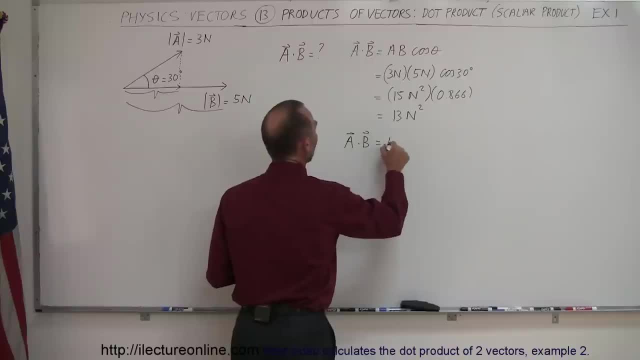 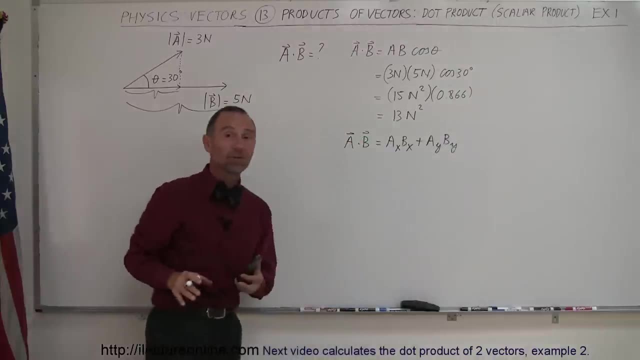 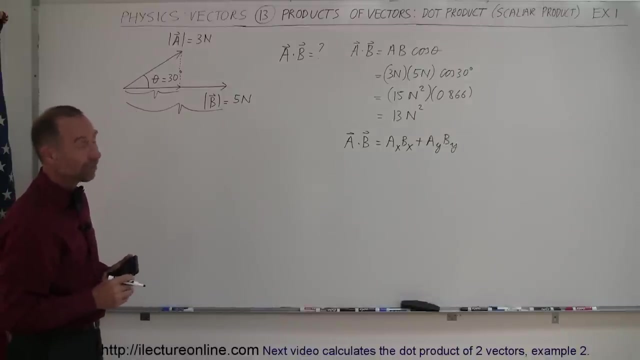 saying that A dot B is equal to AXBX plus AYBY. In other words, we multiply the X components together and we multiply the Y components together, And of course we should get the same answers before 13 newton squared. That's true. So first we have to find the X and Y components. So A sub X is equal to A times the cosine of 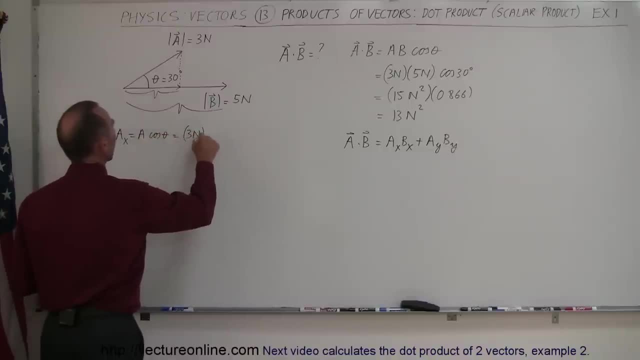 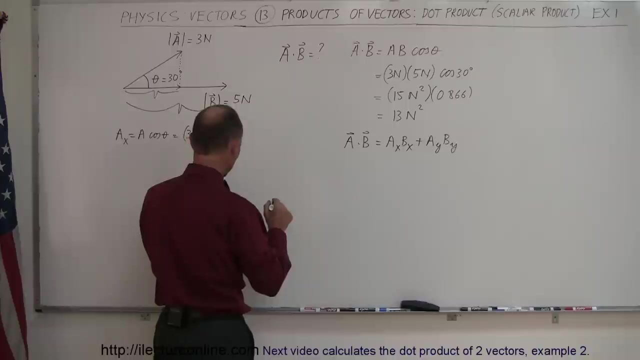 theta, which is equal to 3 newtons times the cosine of 30 degrees. And let's see what that is: equal to 0.866.. I should just go more accurately: 30 cosine times 3 equals, let's say that's 20, that's 2.598.. 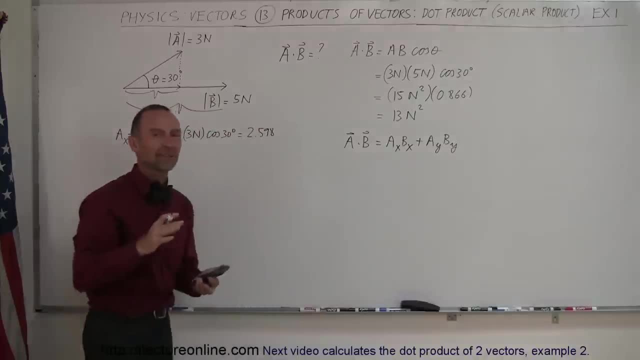 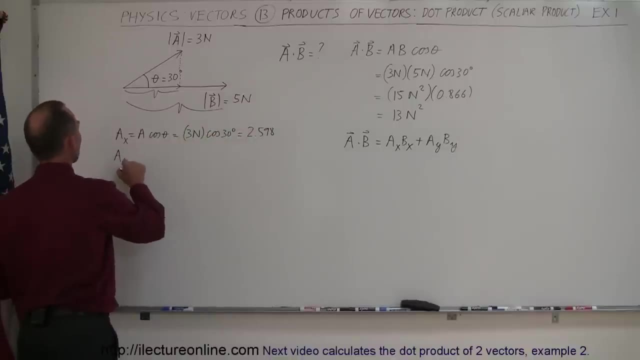 So 2.598.. I'm keeping a lot of significant figures- Actually they're not that significant, but just to make sure I get about the same answers before. So we have A sub Y which is equal to A times the cosine. Oh, not the cosine, I'm looking for the.